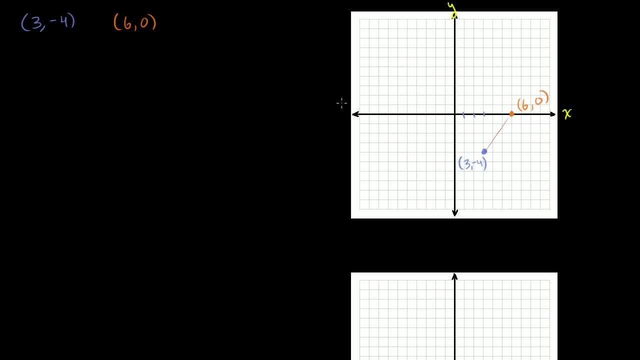 I don't see a triangle there, And if you don't see a triangle, let me draw it for you. Let me draw the triangle, Let me draw this triangle right there, just like that. Let me actually do several colors here, just to really. 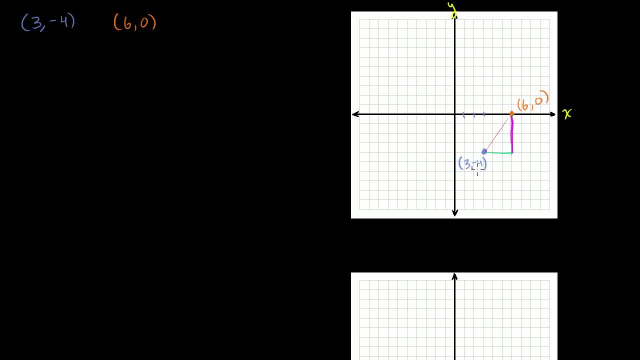 hit the point home. So there's our triangle And you might immediately recognize this is a right triangle. This is a right angle. right there The base goes straight left to right. The right side goes straight up and down, So we're dealing with a right triangle. 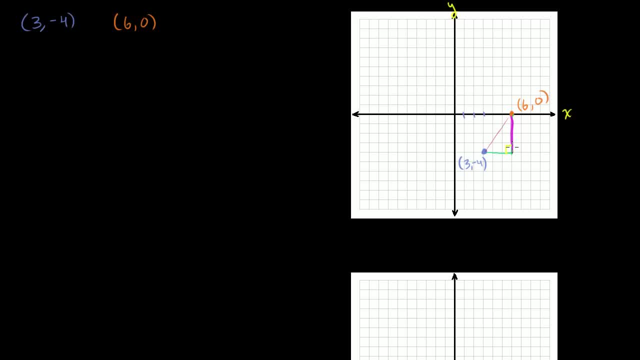 So if we could just figure out what the base length is and what this height is, we could use the Pythagorean theorem to figure out this long side, the side that is opposite, the right angle, the hypotenuse This. right here, the distance is the hypotenuse of this. 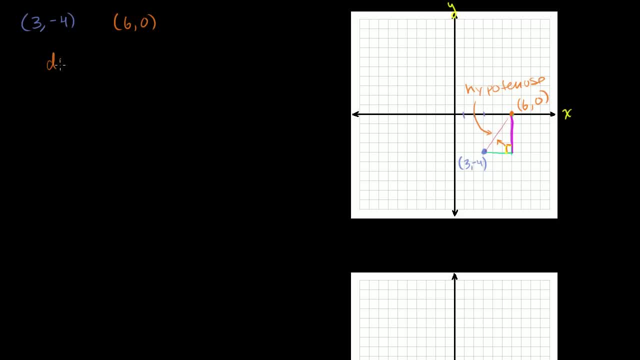 right triangle. Let me write that down. The distance is equal to the hypotenuse of this right triangle, So let me draw it a little bit bigger. So this is the hypotenuse right there, And then we have the side on the right, the side that goes. 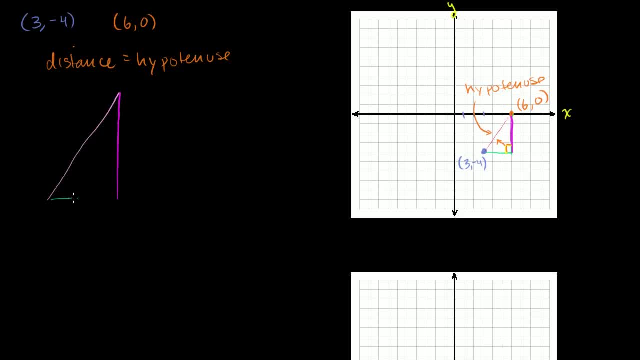 straight up and down And then we have our base. Now how do we figure out- Let's call this d for distance, That's the length of our hypotenuse. How do we figure out the lengths of this up and down side and the base side right here? 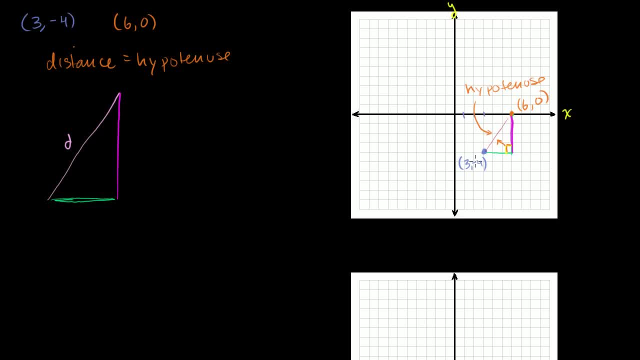 So let's look at the base first. What is this distance? You could even count it on this graph paper. But here we're at: x is equal to 3. And here we're at: x is equal to 6.. We're just moving straight, right. 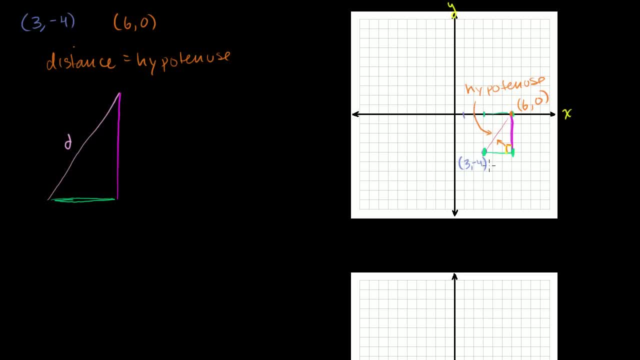 This is the same distance as that distance right there. So to figure out that distance, it's literally the end x point And you can actually go either way because you're going to square everything, so it doesn't matter if you get negative numbers. 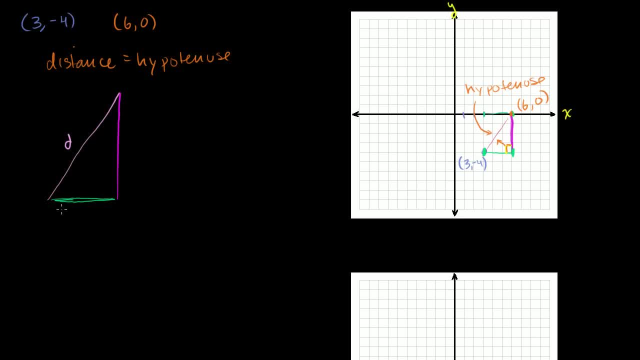 So the distance here is going to be 6 minus 3, right 6 minus 3.. That's this distance right here, which is equal to 3.. So we've figured out the base And just to remind ourselves, that is equal. 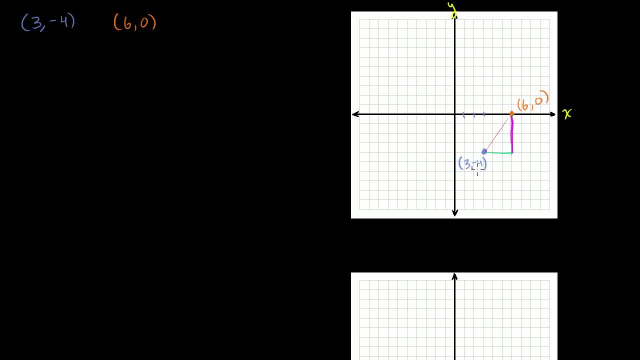 hit the point home. So there's our triangle And you might immediately recognize this is a right triangle. This is a right angle. right there The base goes straight left to right. The right side goes straight up and down, So we're dealing with a right triangle. 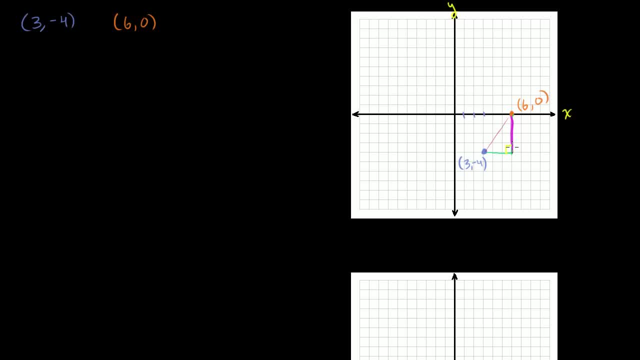 So if we could just figure out what the base length is and what this height is, we could use the Pythagorean theorem to figure out this long side, the side that is opposite, the right angle, the hypotenuse This. right here, the distance is the hypotenuse of this. 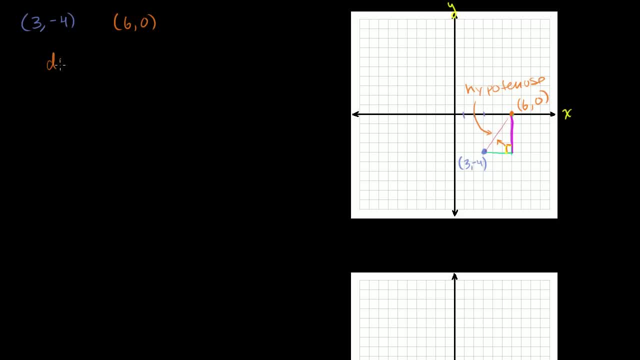 right triangle. Let me write that down. The distance is equal to the hypotenuse of this right triangle, So let me draw it a little bit bigger. So this is the hypotenuse right there, And then we have the side on the right, the side that goes. 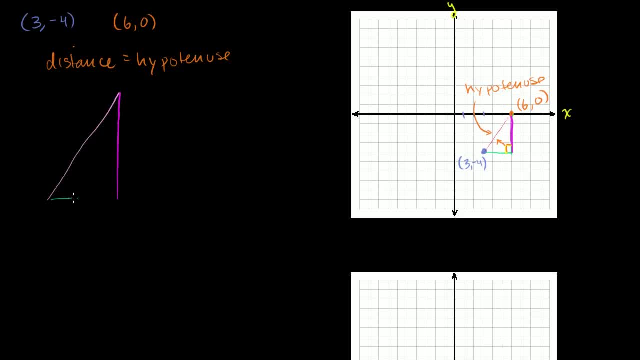 straight up and down And then we have our base. Now how do we figure out- Let's call this d for distance, That's the length of our hypotenuse. How do we figure out the lengths of this up and down side and the base side right here? 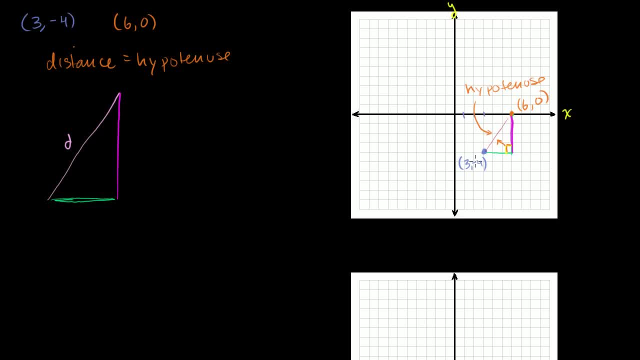 So let's look at the base first. What is this distance? You could even count it on this graph paper. But here we're at: x is equal to 3. And here we're at: x is equal to 6.. We're just moving straight, right. 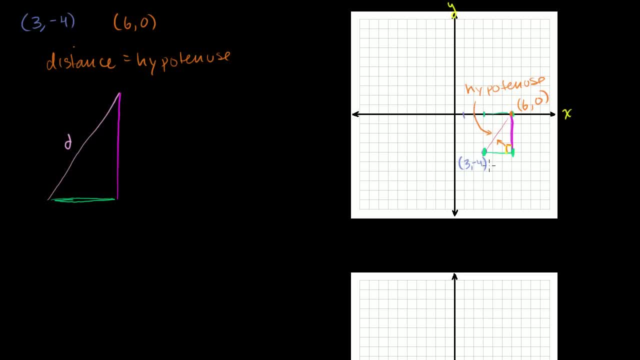 This is the same distance as that distance right there. So to figure out that distance, it's literally the end x point And you can actually go either way because you're going to square everything, so it doesn't matter if you get negative numbers. 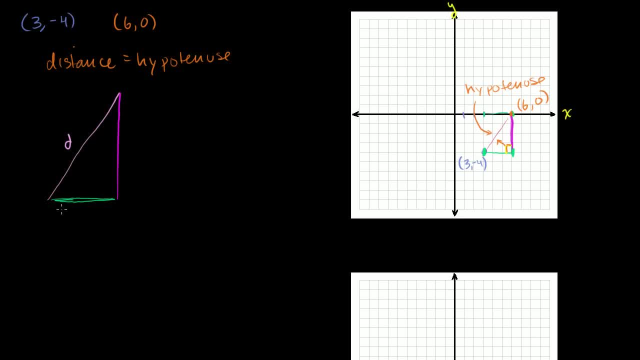 So the distance here is going to be 6 minus 3, right 6 minus 3.. That's this distance right here, which is equal to 3.. So we've figured out the base And just to remind ourselves, that is equal. 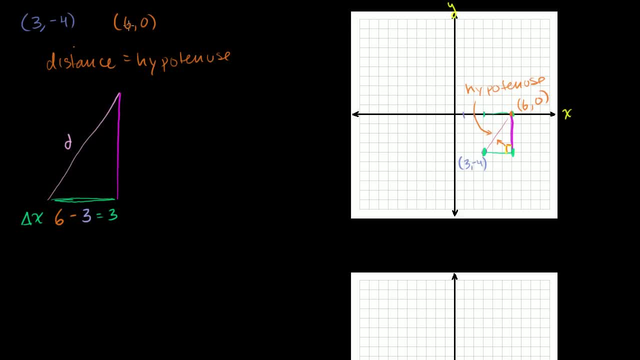 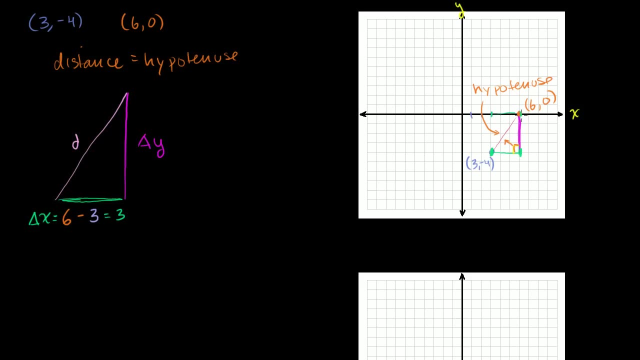 to the change in x. That was equal to your finishing x minus your starting x, 6 minus 3.. This is our delta x. Now, by the same exact line of reasoning, this height right here is going to be your change in y. 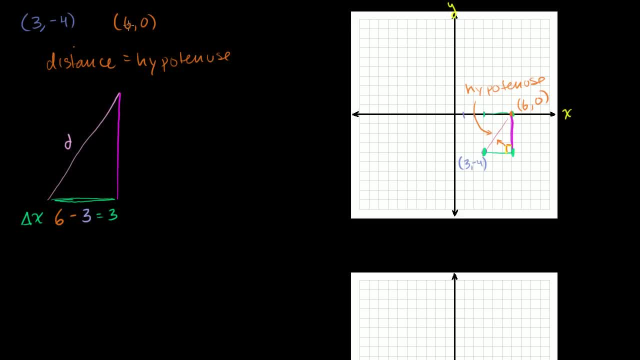 to the change in x. That was equal to your finishing x minus your starting x, 6 minus 3.. This is our delta x. Now, by the same exact line of reasoning, this height right here is going to be your change in y. 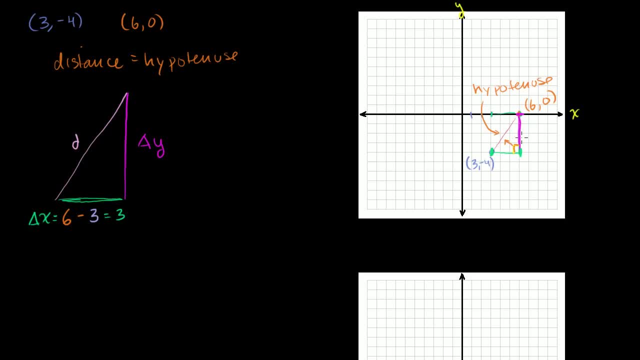 Up here you're at. y is equal to 0.. That's kind of where you finish. That's your higher y point, And over here you're at. y is equal to negative 4.. So change in y is equal to 0 minus negative 4.. 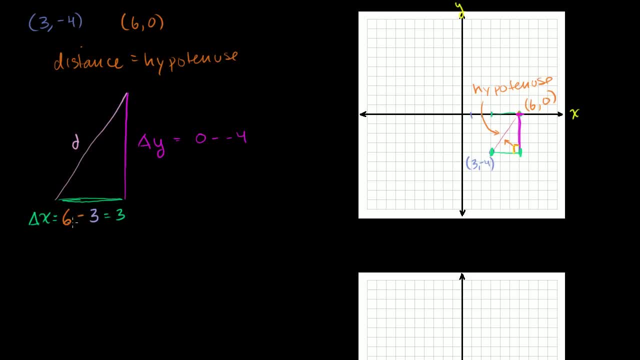 I'm just taking the larger y value minus the smaller y value, The larger x value minus the smaller x value. But you're going to see, We're going to square it in a second. so even if you did it the other way around, 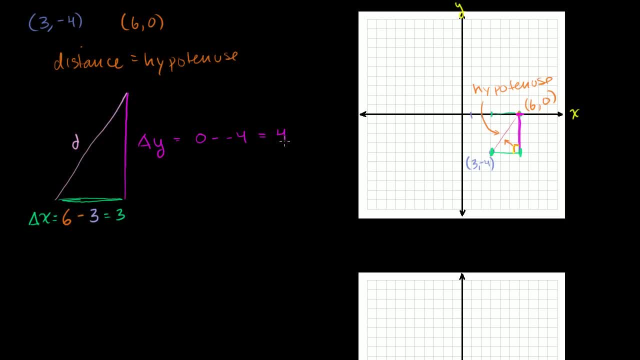 You get a negative number, but you still get the same answer. So this is equal to 4.. So this side is equal to 4.. You could even count it on the graph paper if you like. And this side is equal to 3.. 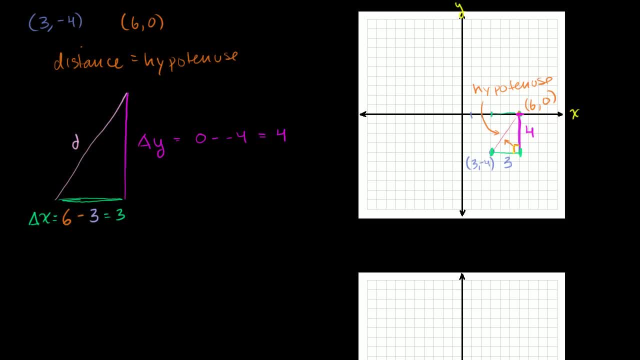 And now we can do the Pythagorean theorem. This distance is the distance squared. Be careful: The distance squared is going to be equal to this delta x squared: the change in x squared plus the change in y squared plus the change in y squared. 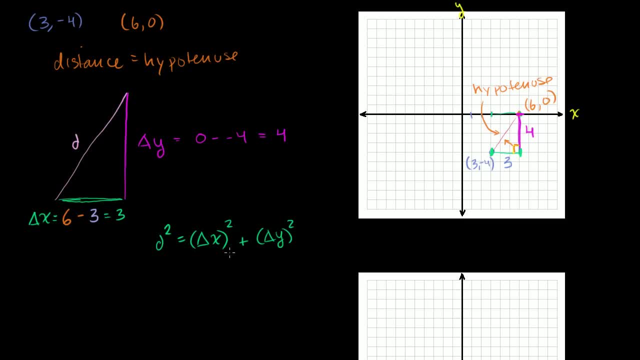 This is nothing fancy. Sometimes people will call this the distance formula. It's just the Pythagorean theorem: This side squared plus that side squared is equal to hypotenuse squared, because this is a right triangle. So let's apply it with these numbers, the numbers that we 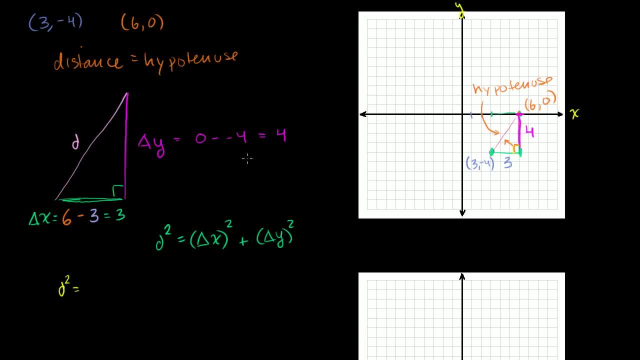 have at hand. So the distance squared is going to be equal to: delta x squared is 3 squared, Plus delta y squared plus 4 squared, which is equal to 9 plus 16, which is equal to 25.. So the distance is equal to. let me write that: 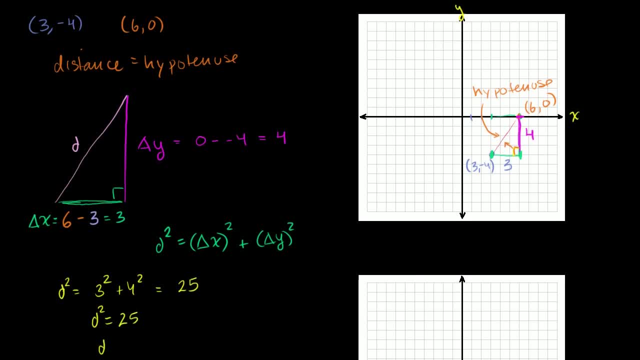 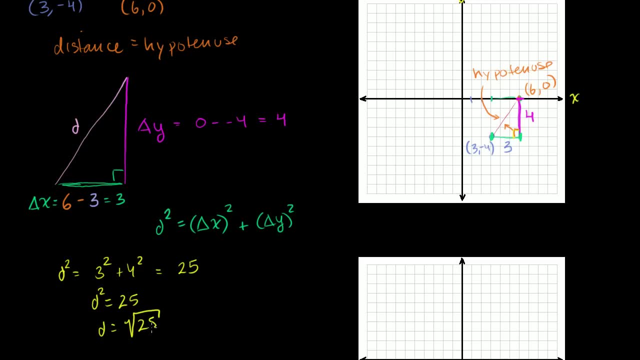 d squared is equal to 25.. d, our distance is equal to you. don't want to take the negative square root because you can't have a negative distance, so only the principal root, the positive square root of 25, which is equal to 5.. 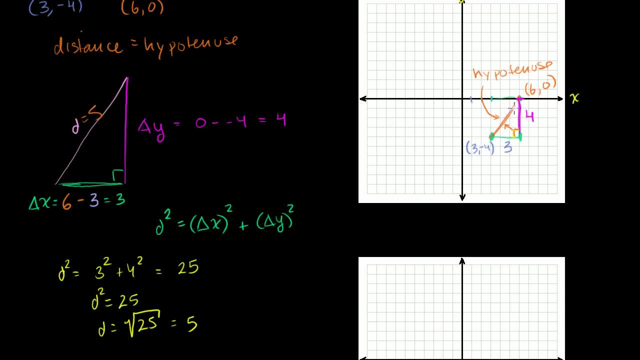 So this distance right here is 5.. Or if we look at this distance right here, that was the original problem- How far is this point from that point? It is 5 units away. So what you'll see here, they call it the distance formula. 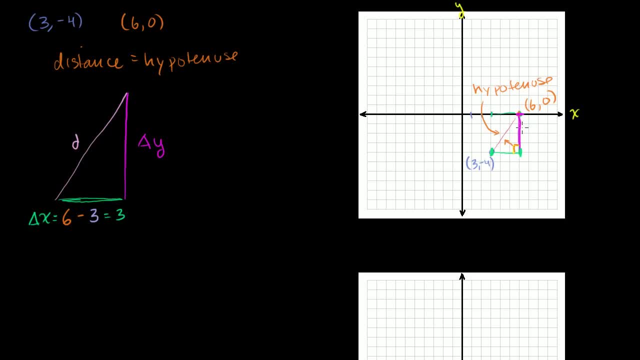 Up here you're at. y is equal to 0.. That's kind of where you finish. That's your higher y point, And over here you're at. y is equal to negative 4.. So change in y is equal to 0 minus negative 4.. 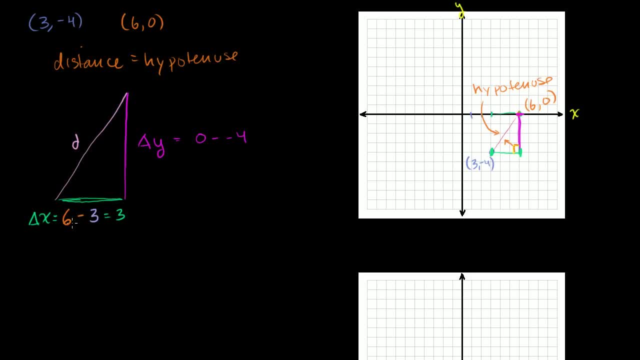 I'm just taking the larger y value minus the smaller y value, the larger x value minus the smaller x value. But you're going to see, we're going to square it in a second, So you might get it the other way around: You get a negative number but you still get the same answer. 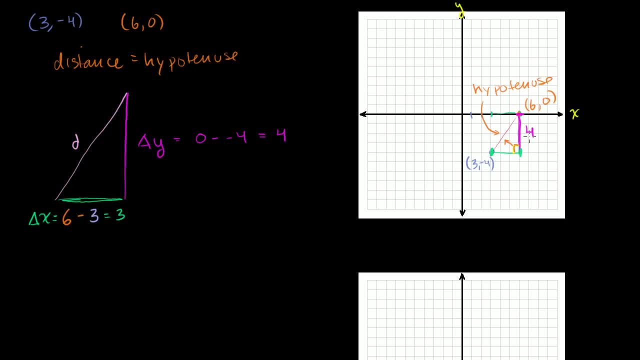 So this is equal to 4.. So this side is equal to 4.. You could even count it on the graph paper, if you like. And this side is equal to 3.. And now we can do the Pythagorean theorem. This distance is the distance squared. 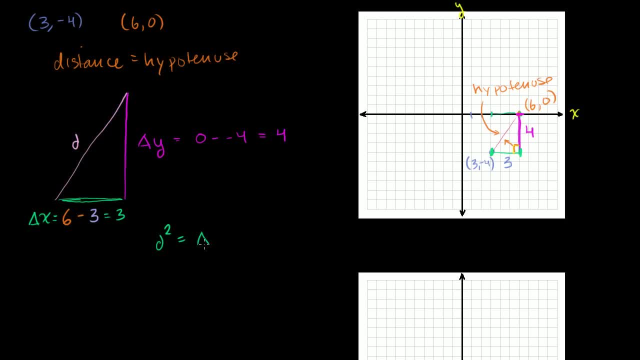 Be careful. The distance squared is going to be equal to this: delta x squared, the change in x squared plus the change in y squared plus the change in y squared. This is nothing fancy. Sometimes people will call this the distance formula. 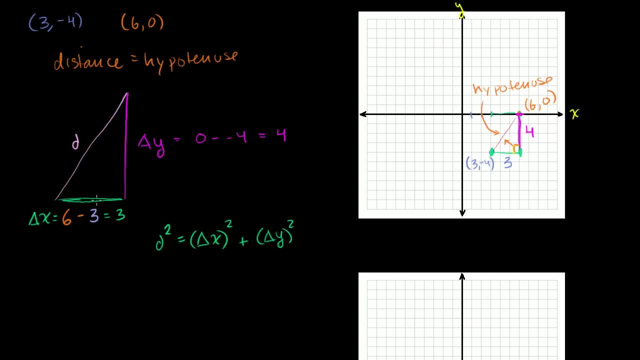 It's just the Pythagorean theorem. This side squared plus that side squared is equal to hypotenuse squared, because this is a right triangle. So let's apply it with these numbers, the numbers that we have at hand. So the distance squared is going to be equal to delta x. 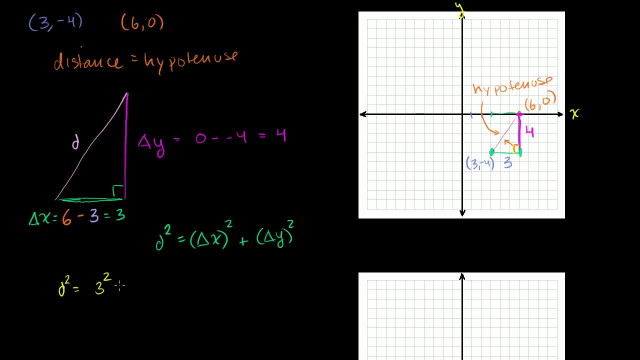 squared is 3 squared plus delta, y squared plus 4 squared, which is equal to 9 plus 16. Which is equal to 25.. So the distance is equal to. let me write that d squared is equal to 25.. 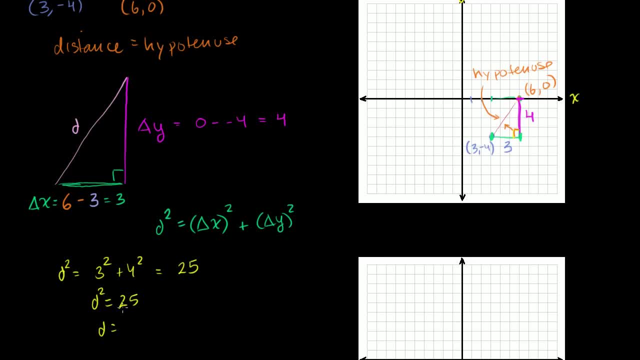 d, our distance is equal to. you. don't want to take the negative square root because you can't have a negative distance, so only the principal root, the positive square root of 25, which is equal to 5.. So this distance right here is 5.. 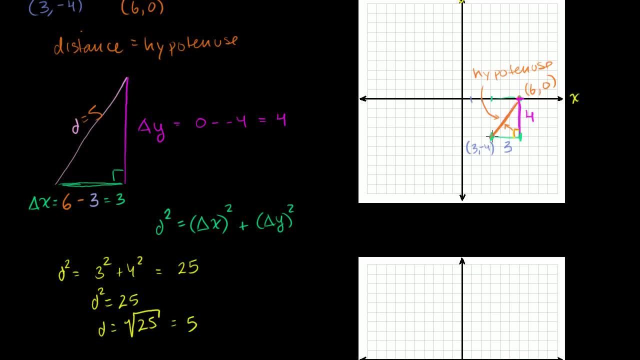 Or if we look at this distance right here- that was the original problem- How far is this point? from that point It is 5 units away, But you'll see here. they call it the distance formula, but it's just the Pythagorean theorem. 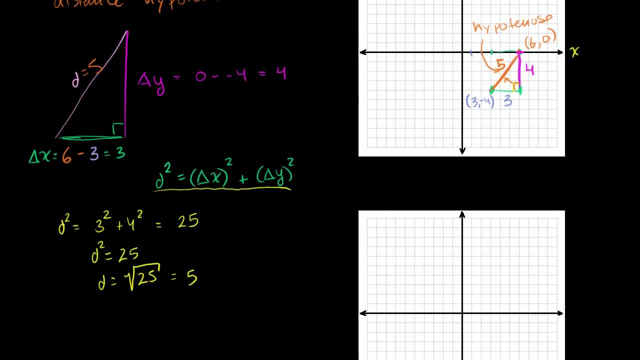 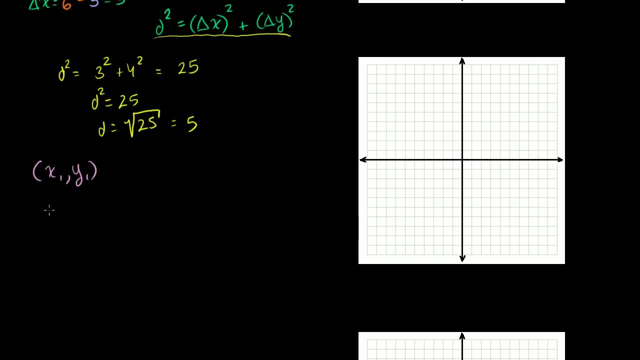 And just so you're exposed to all of the ways that you'll see the distance formula. sometimes people will say, oh, if I have two points, if I have one point, let's call it x1 and y1.. So that's just a particular point. 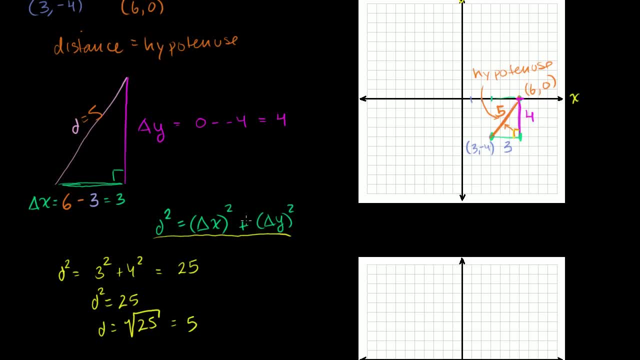 but it's just the Pythagorean theorem, And just so you're exposed to all of the ways that you'll see the distance formula. sometimes people will say, oh, if I have two points, if I have one point, let's call it. 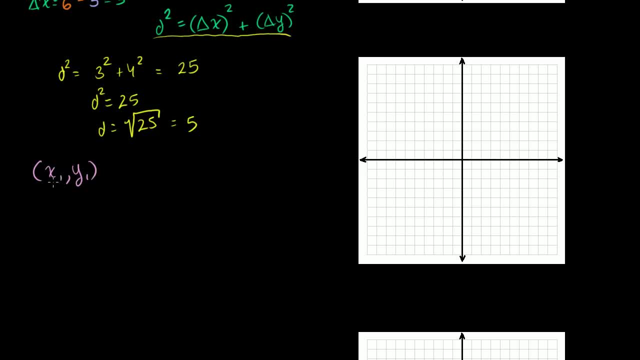 x1 and y1.. So that's just a particular point. And let's say I have another point, that is, x2 comma y2.. Sometimes you'll see this formula that the distance of x1 and x2 at a distance. You'll see it in different ways, but you'll see that the 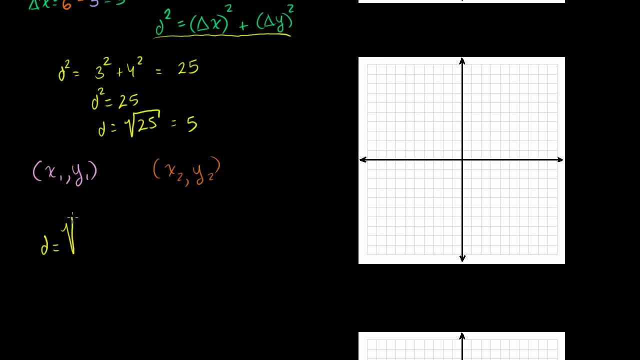 distance is equal to: and this looks like a really complicated formula, but I want you to see that this is really just a Pythagorean theorem. You see that the distance is equal to x2 minus x1 squared, plus y2 minus x2 squared. 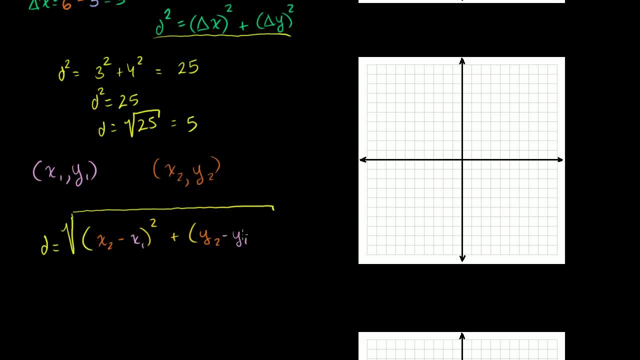 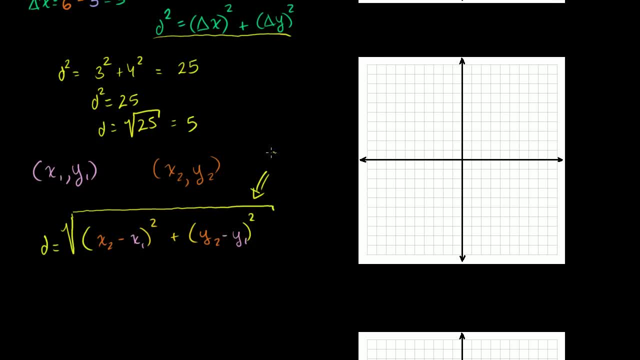 You'll see this written in a lot of textbooks as the distance formula, And it's a complete waste of your time to memorize it, because it's really just the Pythagorean theorem. This is your change in x, And it really doesn't matter which x you pick to be first. 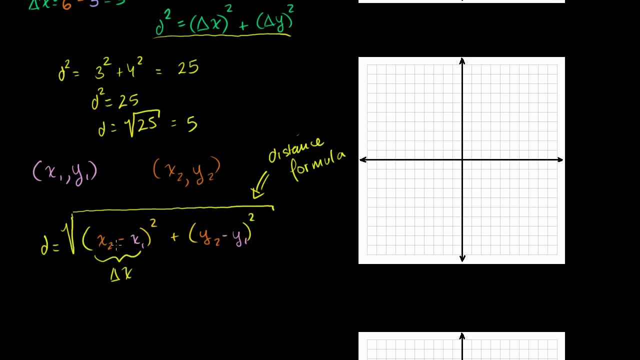 or second, because even if you get the negative of this value, when you square it, the negative disappears. This, right here, is your change in y. So it's just saying that the distance squared. remember, if you square both sides of this equation, the radical will. 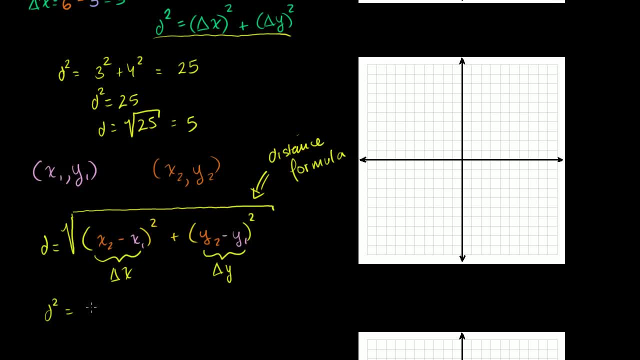 disappear and this will be the distance. squared is equal to this expression. squared delta x squared. change in x. Delta means change in Delta x squared plus delta y squared. Don't want to confuse you. Delta y just means change in y. 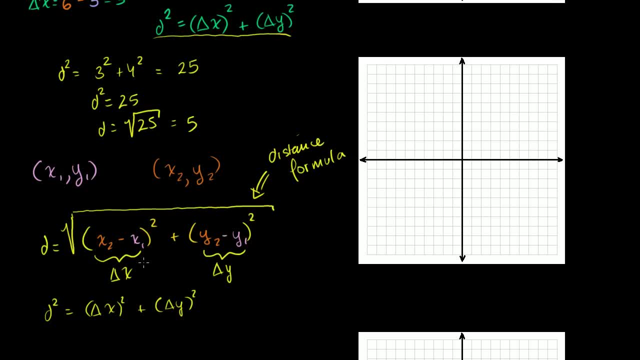 I should have probably said that earlier in the video, But let's apply it to a couple of more And I'll just pick some points at random. Let's say I have the point. let's see 1,, 2,, 3,, 4,, 5, 6,. 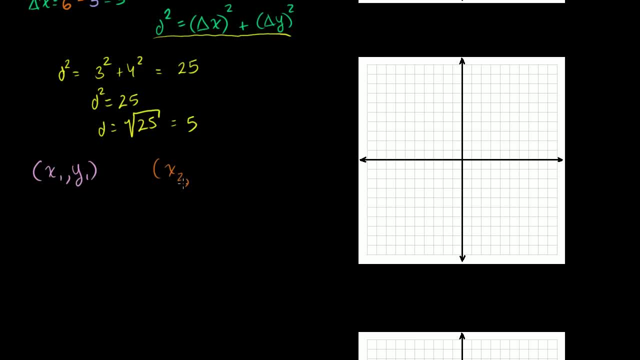 And let's say I have another point, that is, x2 comma y2.. Sometimes you'll see this formula that the distance- you'll see it in different ways, but you'll see that the distance is equal to It- looks like this: 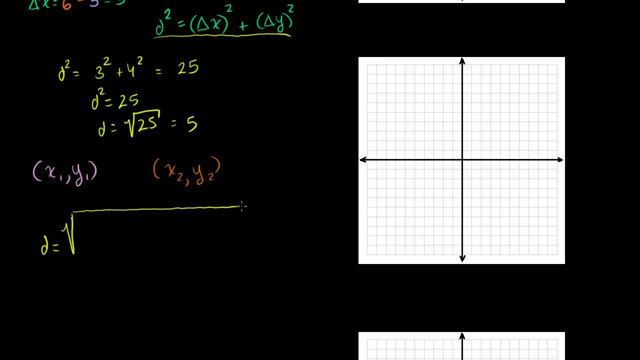 Really complicated formula, but I want you to see that this is really just the Pythagorean theorem. You'll see that the distance is equal to x2 minus x1 squared, plus y2 minus y1 squared. You'll see this written in a lot of textbooks. 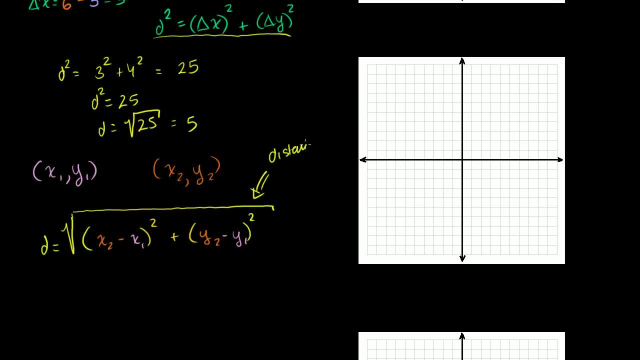 As the distance formula, And it's a complete waste of your time to memorize it, because it's really just the Pythagorean theorem. This is your change in x, And it really doesn't matter which x you pick to be first or second, because even if you get the negative of this value, 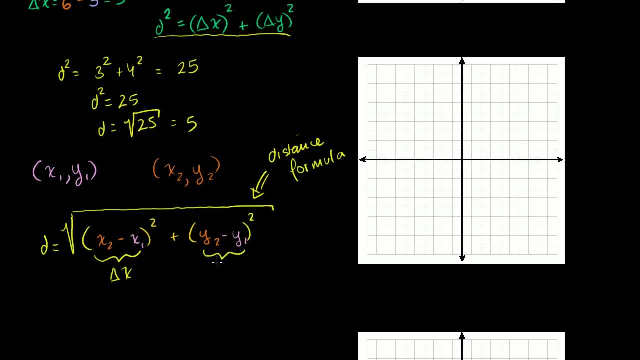 when you square it, the negative disappears. This, right here, is your change in y. So it's just saying that the distance squared. Remember, if you square both sides of this equation, the radical will disappear and this will be the distance. 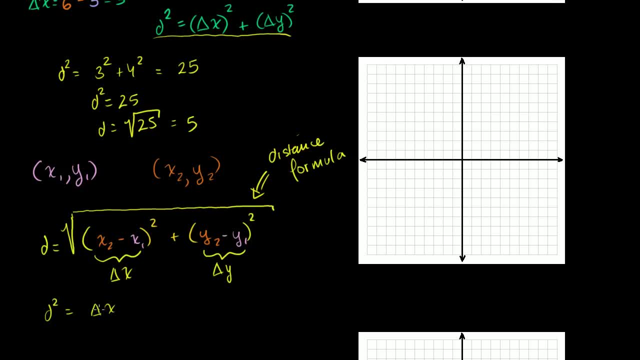 squared is equal to this expression: squared delta x squared. change in x. Delta means change in Delta x squared plus delta y squared. Don't want to confuse you. Delta y just means change in y. I should have probably said that earlier in the video. 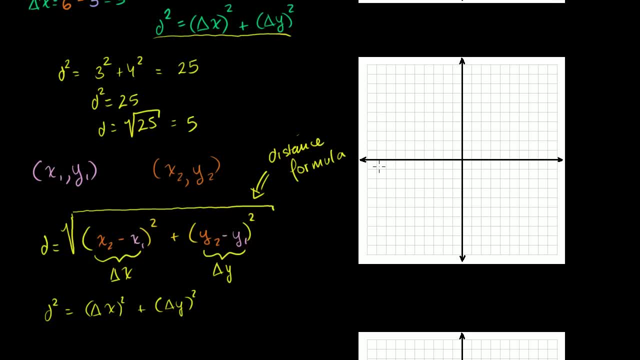 But let's apply it to a couple of more And I'll just pick some points at random. Let's say I have the point. let's see 1,, 2, 3, 4, 5, 6.. 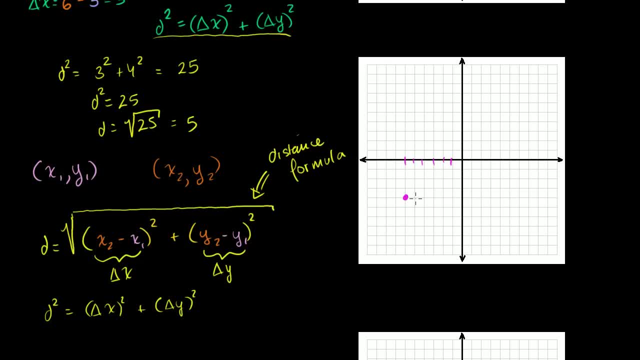 Negative: 6 comma negative: 4.. And let's say, I want to find the distance between that and 1 comma 1,, 2,, 3,, 4,, 5,, 6,, 7.. And the point 1 comma 7.. 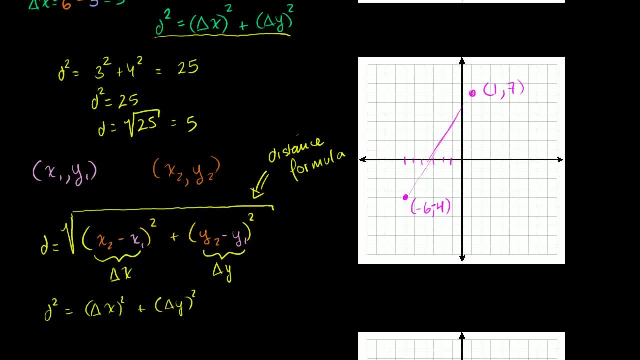 So I want to find this distance right here. So it's the exact same idea. We just use the Pythagorean theorem. You figure out: this distance which is our change in x, This distance which is our change in y, This distance squared plus, this distance squared is going: 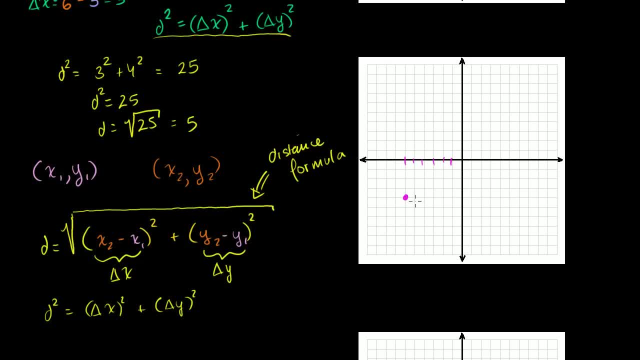 negative 6, negative 4, and let's say, I want to find the distance between that and 1,, 1,, 2,, 3,, 4,, 5,, 6,, 7, and the point 1, 7..